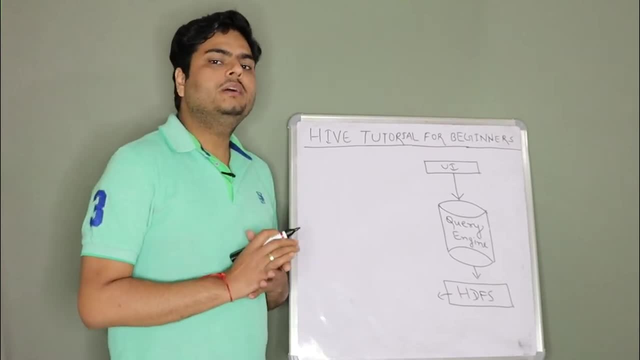 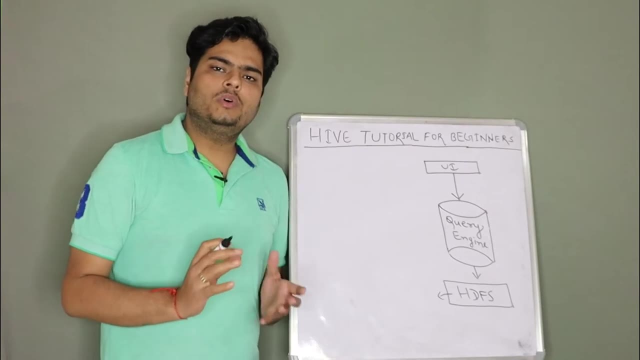 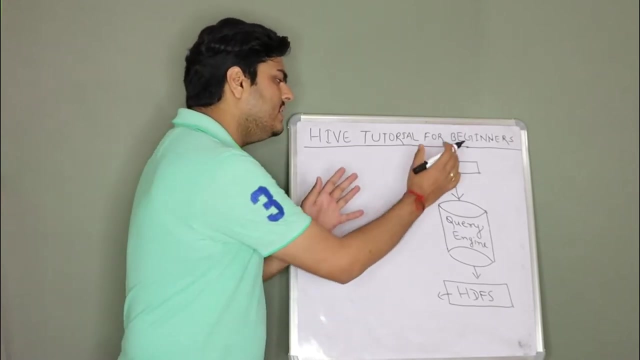 Welcome to Unfold Data Science friends. This is Aman here, and I am a data scientist. In this particular video, we will understand what is Hive, how Hive works and why Hive is so popular among data scientists. I am also going to explain you some basic architecture of Hive. 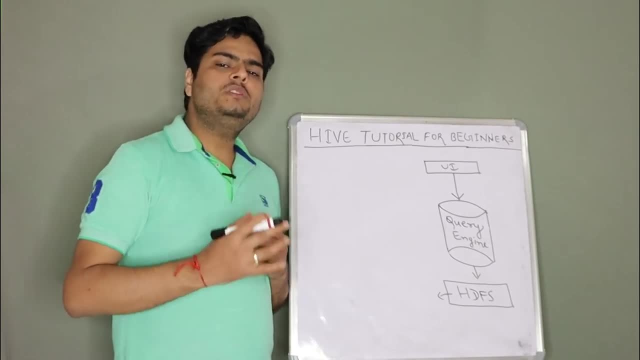 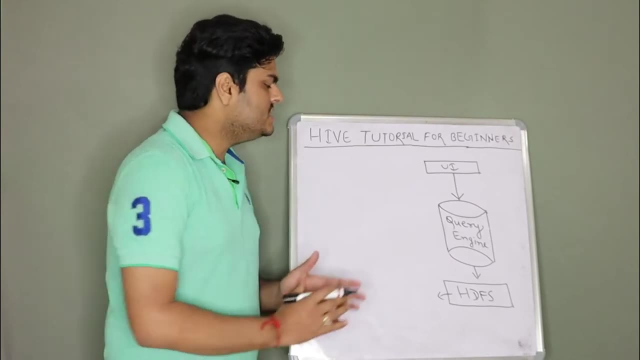 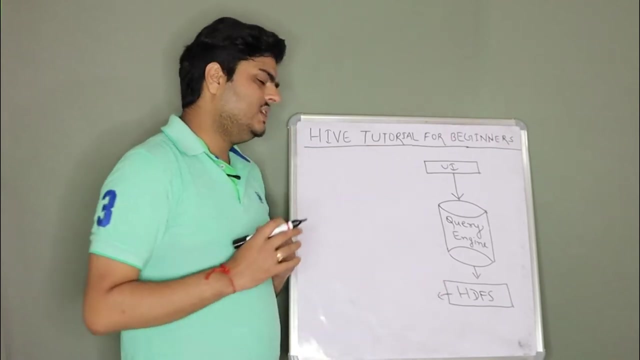 what are some pros and cons of Hive and why Hive is used. All these things we will know in this video. Let us start one by one. First of all, guys, what is Hive? So I have already explained you in my previous videos in this same playlist. what is HDFS, right? So HDFS is nothing but. 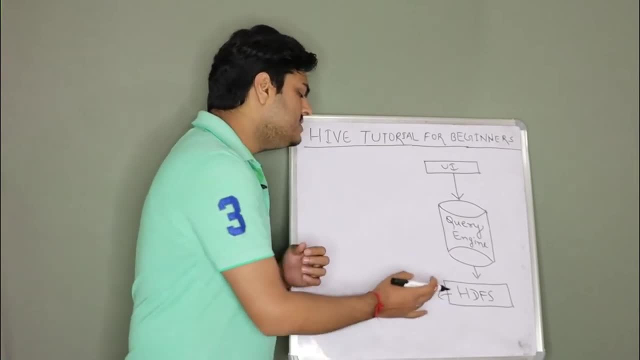 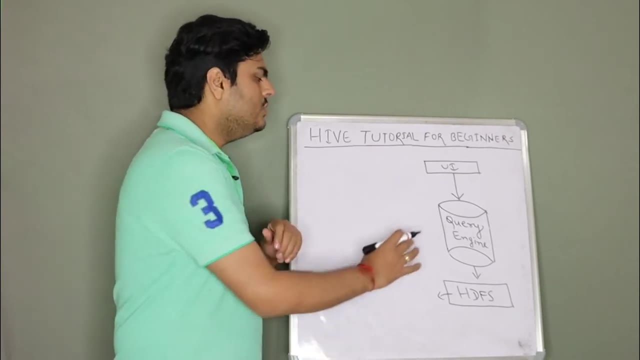 Haroop Distributed File System. So this is a file system based on Haroop ecosystem, So the way files are stored in Haroop- okay. Now what is Hive, guys? So this is basically architecture of Hive that you are seeing here. What is Hive? Hive is. 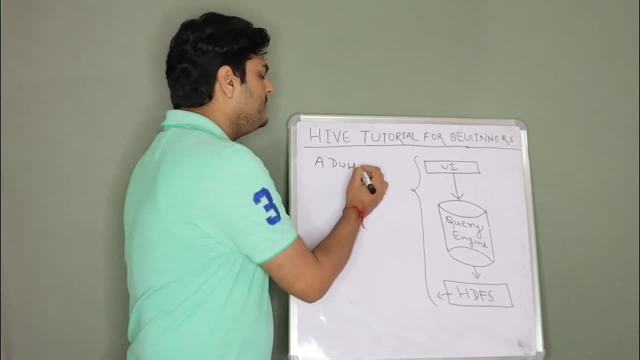 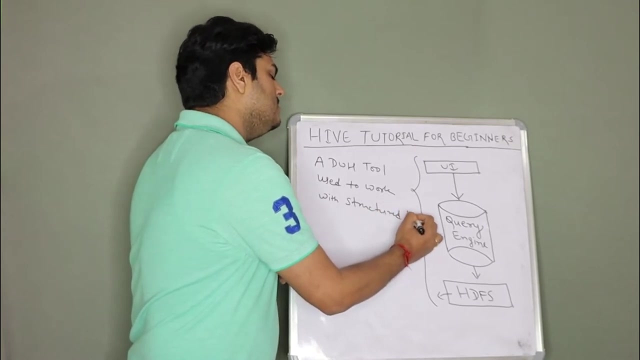 nothing but a data warehouse tool. okay, Data warehouse tool used to work with- used to work with- structured data? okay, Structured data. Now some of you might be thinking: what is data warehouse tool? So data warehouse is a very simple concept, guys to. 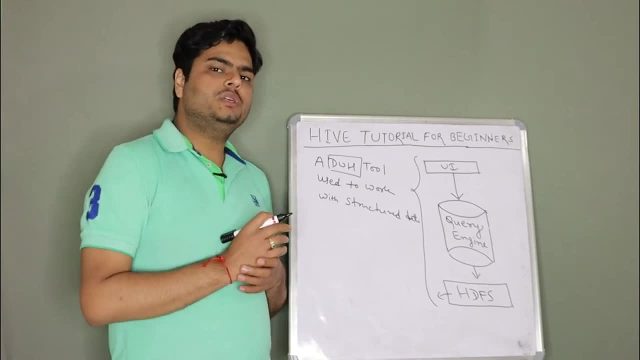 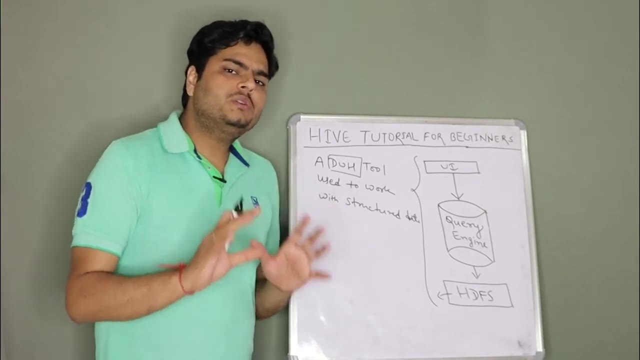 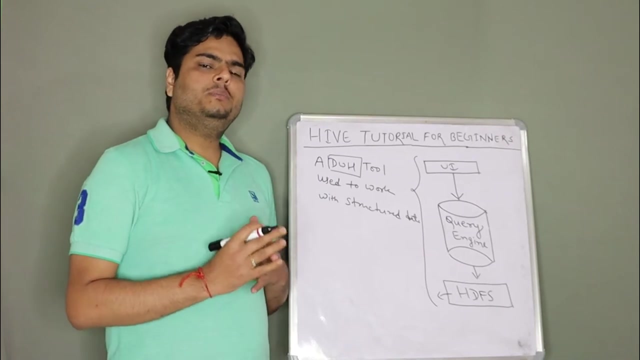 understand for some of you who is not aware of what data warehouse is. Let us say, in your home also, you might be having a store kind of area right Where you put something which you do not use very regularly. So data warehouse is also same concept. So if you take example of, let us 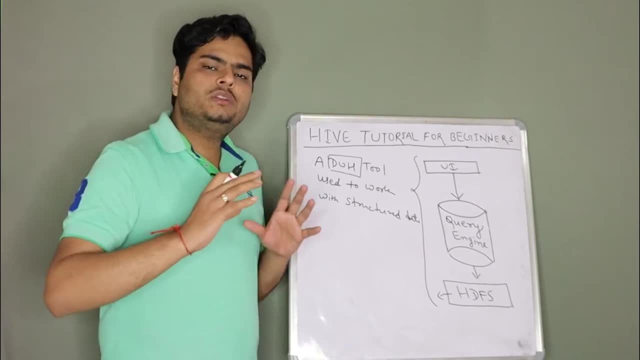 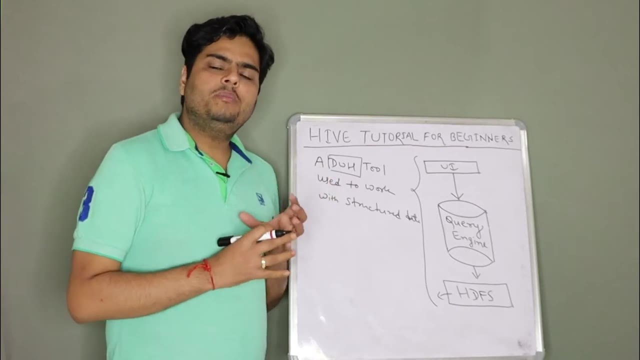 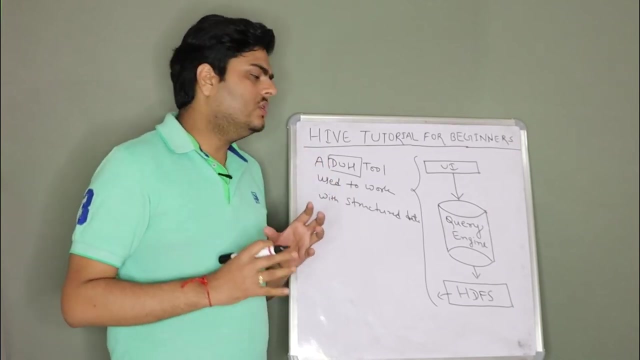 say, pantalons or big bazaar or, let us say, any other retail store. all these guys will have some transactional data, right? But all these old transactional data they might not be using in day-to-day basis, right? So all this data they will push in a system. That system is called data. 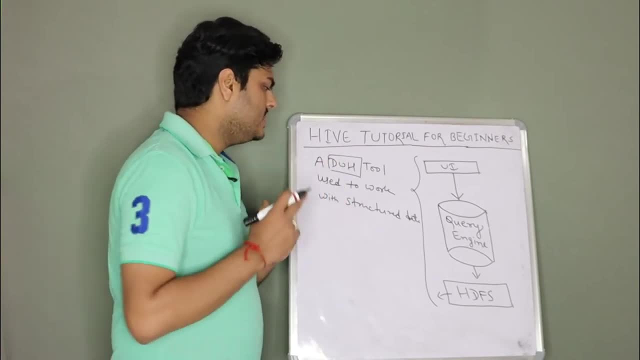 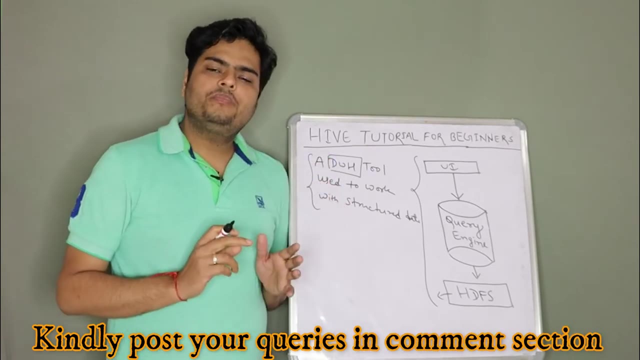 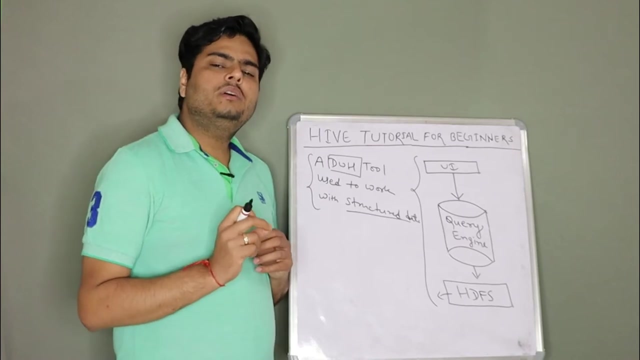 warehouse. All the historical data will be stored in data warehouse. okay, So Hive is used for data warehousing tool on top of Hadoop, okay, And basically with structured data. What I mean by structured data, guys? Structured data is nothing but a data which you can store in the form of 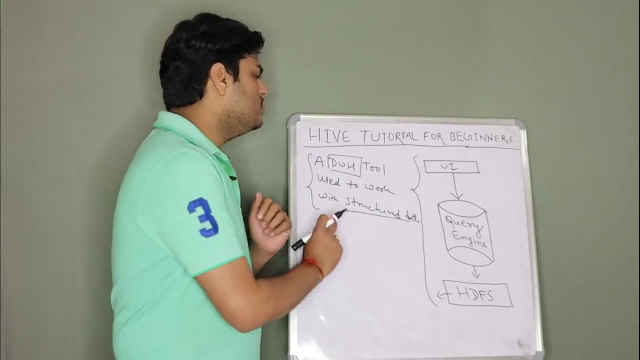 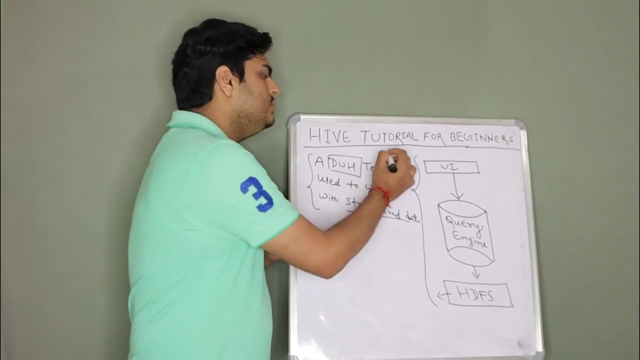 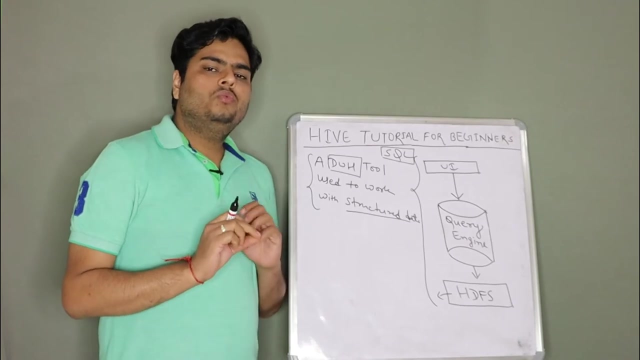 rows and columns. okay, Now why Hive is so popular is most of you, or most of us, are very, very familiar with SQL, right Structured query language. We are very familiar with SQL, and anywhere we see data, we want to retrieve the data using SQL. We want to do some basic analysis using SQL. 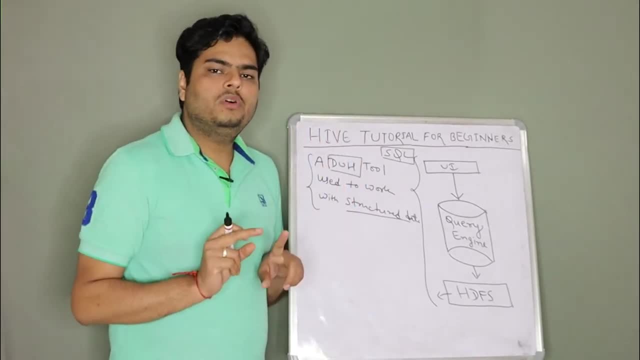 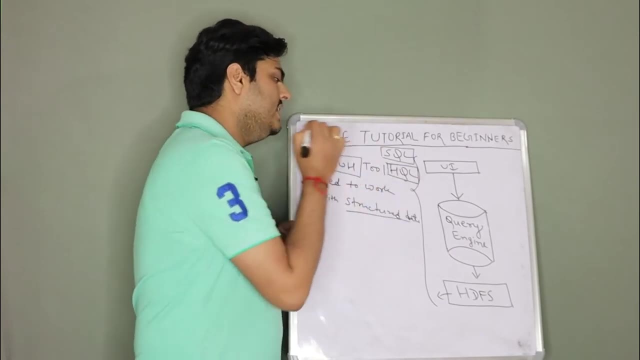 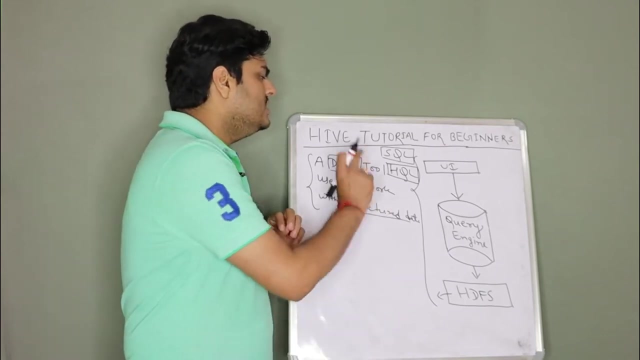 Hive provides you that interface on top of Hadoop. okay, And the language which is used here is called SQL. SQL is standing for Hive query language. SQL is very similar to SQL, almost similar, just few basic differences. So the way you write SQL query, select employee ID, employee name from employee, where some 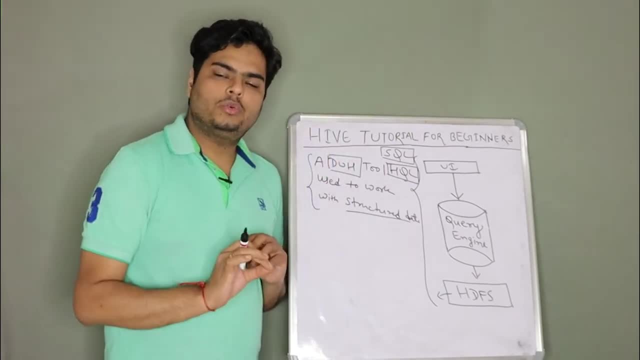 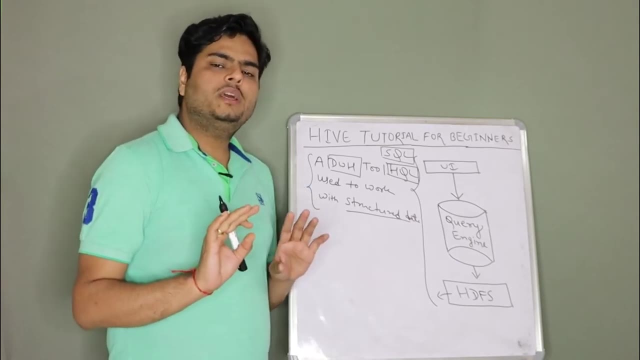 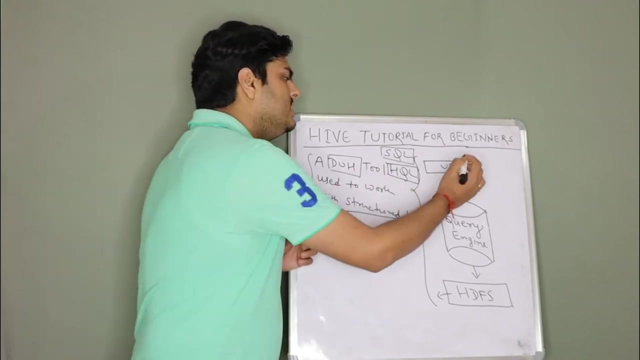 condition: same way, you write a SQL query also. okay, All the people, whether it's a data analyst or data scientist or a big data engineer, all of us can very well analyze the data using this tool. okay, How Hive will work internally. User will come and submit a query here. okay. 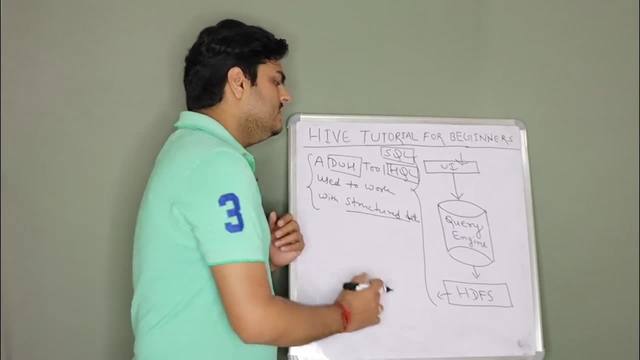 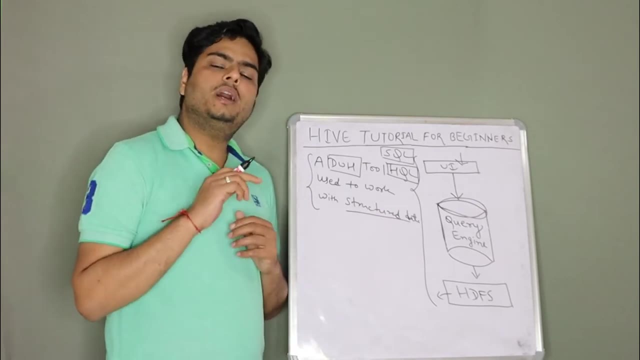 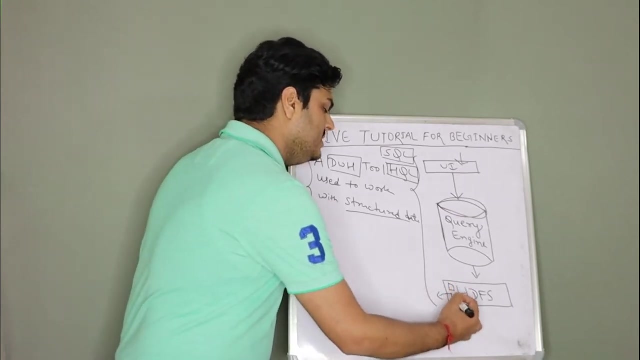 Query means some SQL query. you can say In this query engine, this query will be taken and data- data of the Hive tables is actually stored in form of files in HDFS. So in HDFS you will see different files for different Hive. 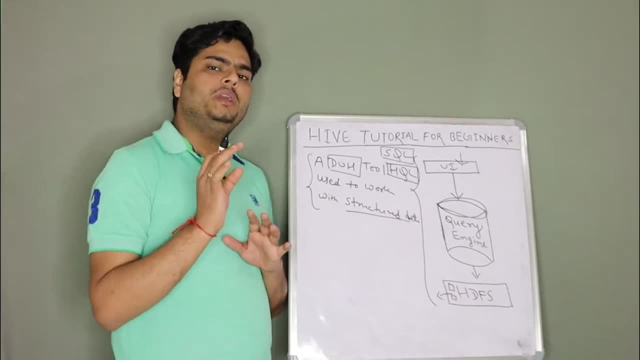 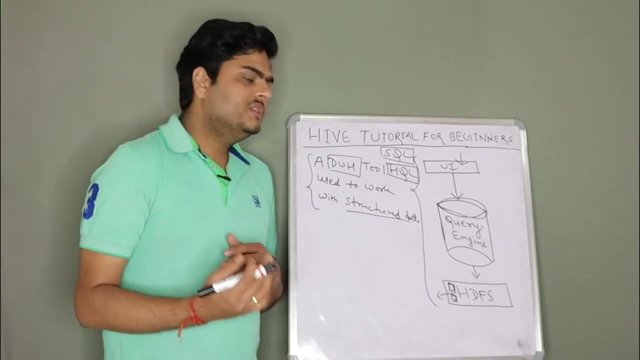 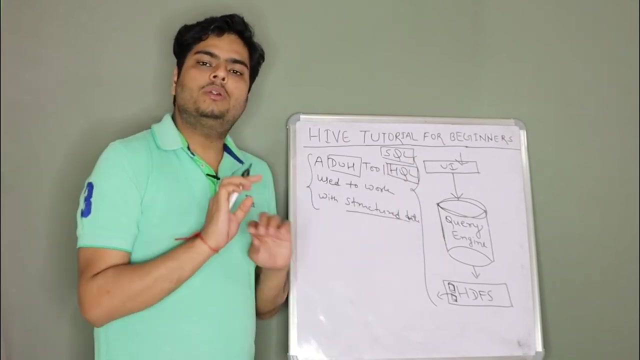 tables. okay. For example, when you say select star from EMP, there will be a table, or there will be a file or many files of EMP data in the HDFS. This query engine will fetch the relevant data from the HDFS And display you the output in the tabular format. All these things we will see in our 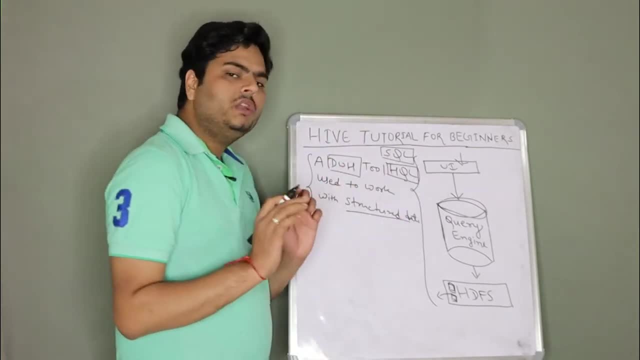 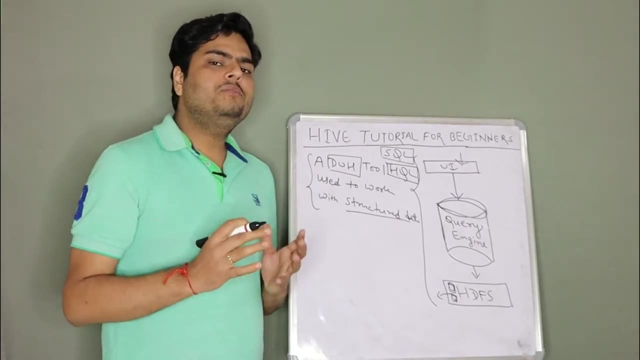 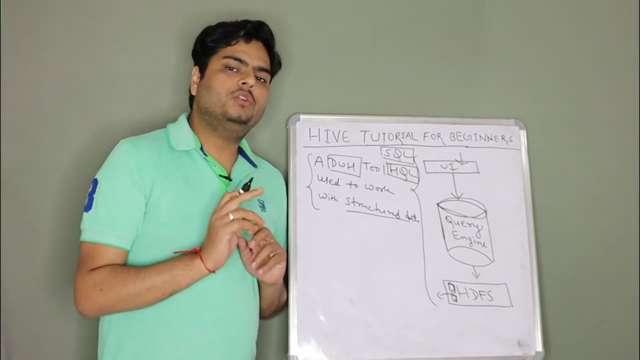 demo guys, don't worry okay. So in the UI you write query and you see the output in a nice tabular format. But internally data is stored in HDFS systems. What Hive can do and what Hive cannot do, It is very important to understand, First of all, the advantages. 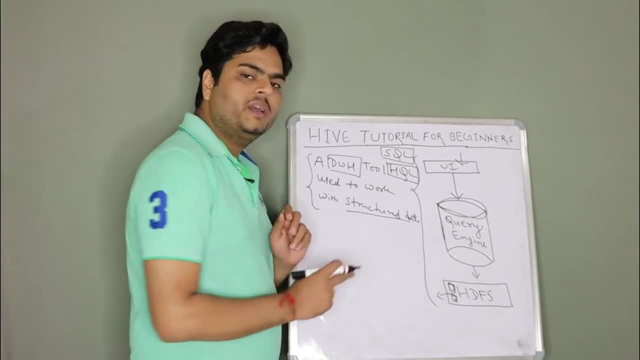 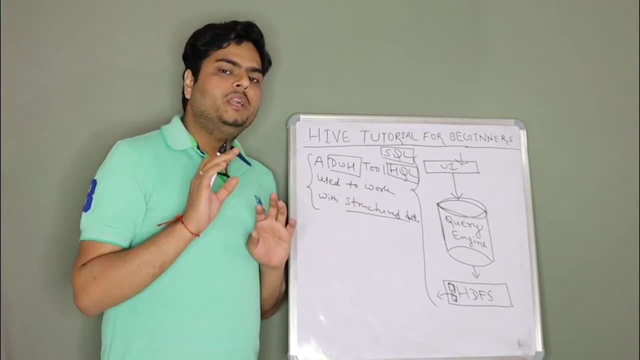 of Hive. okay, So since it uses HDFS in background, hence it can use the advantage of parallel computing. That is the advantage number one. Advantage number two is it will be fast, Since it uses parallel computing, since it uses the power of Haru, hence it will be faster. 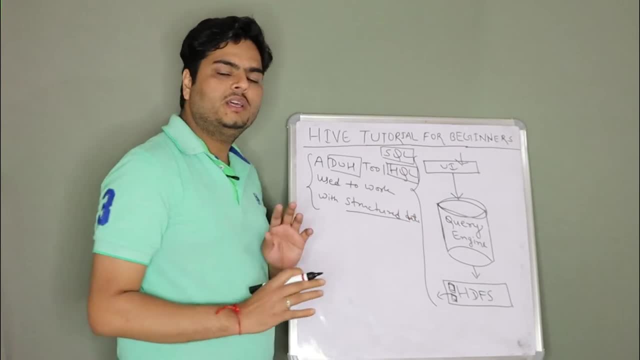 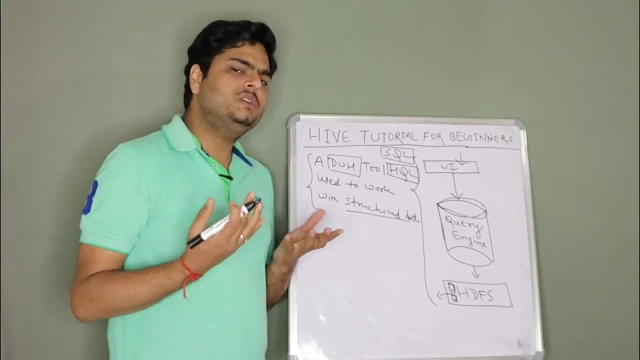 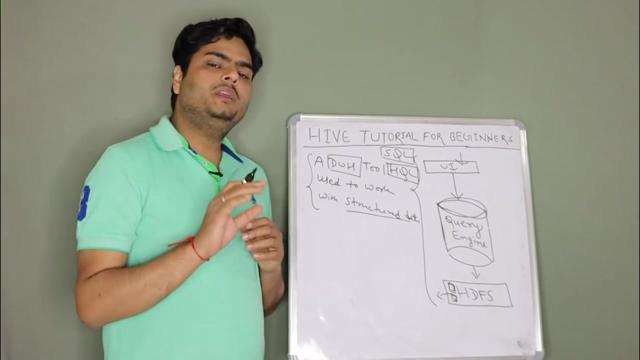 than a normal database if you store huge amount of data, like we store in Hive. Third is: anybody can use it very nicely and easily Because you need to write SQL based queries. Fourth is: Hive is also mounted on top of various cloud offerings, For example in AWS. 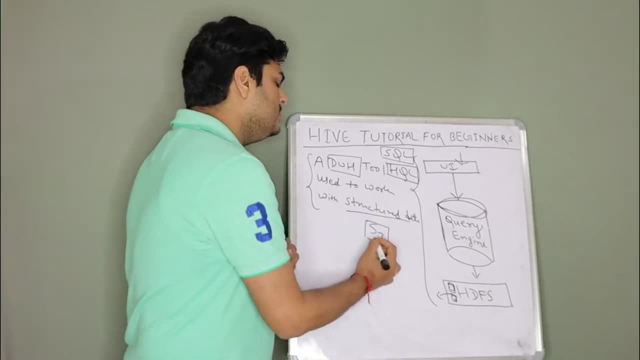 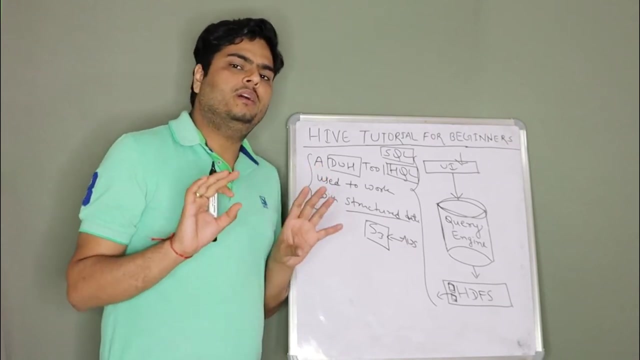 S3.. S3 is a data storage tool on Amazon web services. Here also, you will see, Hive is working in the same way. It works on top of Hadoop. Okay, So Hive is a widely accepted, widely used tool in the world of big data. Okay, Now little bit history of Hive guys. Hive was developed by 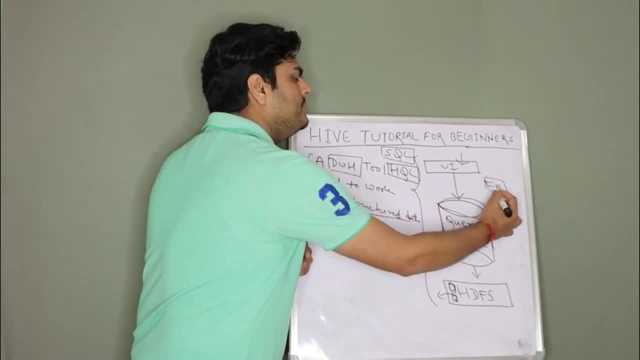 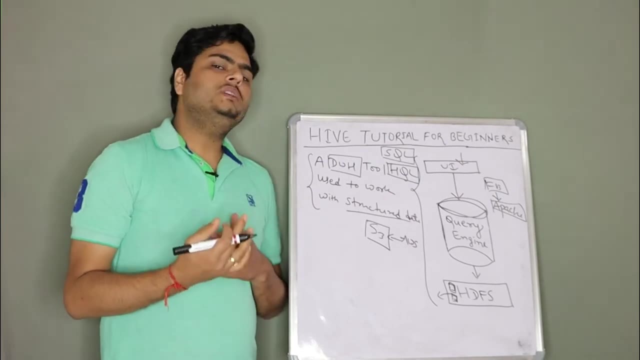 Facebook actually, And then it was taken by Apache and some more features were added, some more advancements were done And now it is known as Apache Hive. Okay, These are about Hive- some of the usability and some of the popularity of Hive. What are the limitations of Hive, guys? 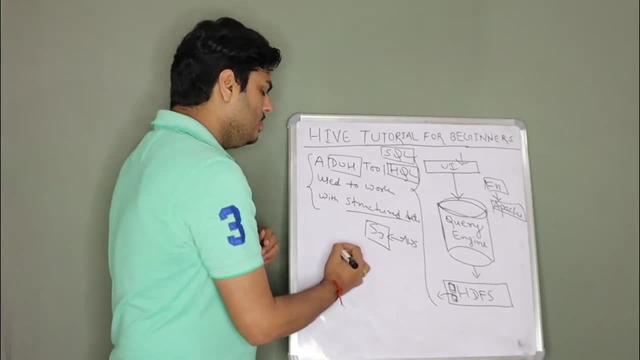 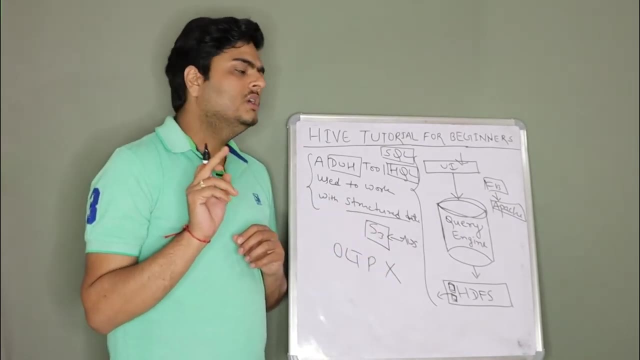 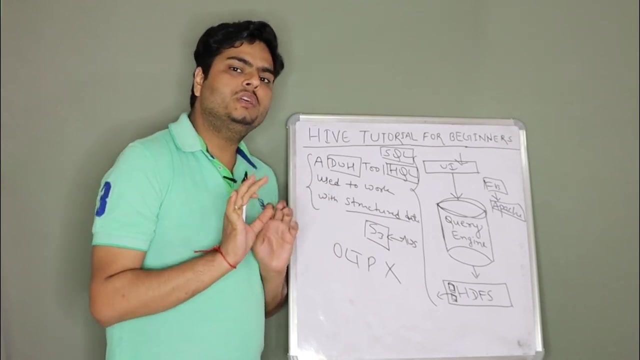 First of all, Hive is not a OLTP system. What is an OLTP system, guys? I was telling you in my Haroop introduction video, also In Hadoop: we cannot process until or unless we are not talking about Spark Kafka, those kind of things. 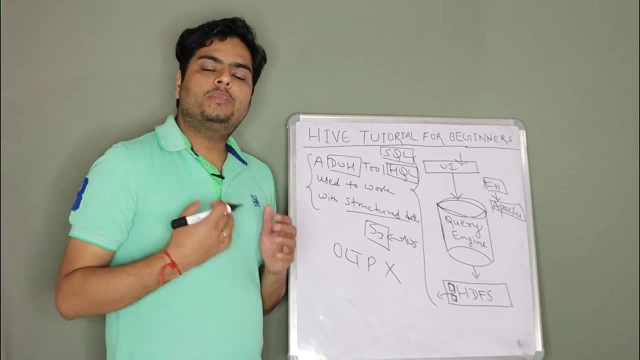 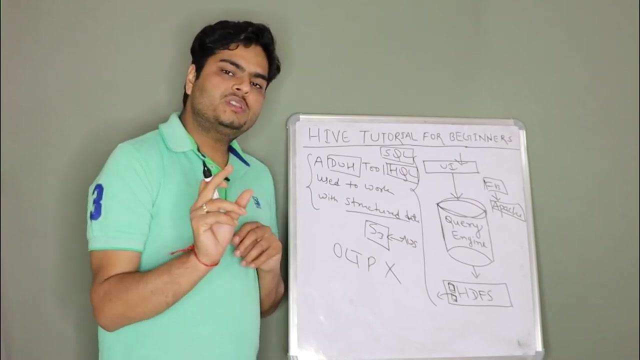 It is not meant for real-time processing. What is meaning by real-time processing? You go to a superstore, you give your card and you tell, hey, can you check if there are some points in my name? So that check has to happen instantly. right, Your card will be scanned and that count of points. 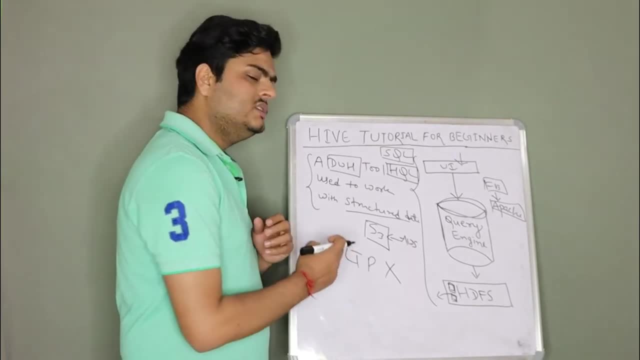 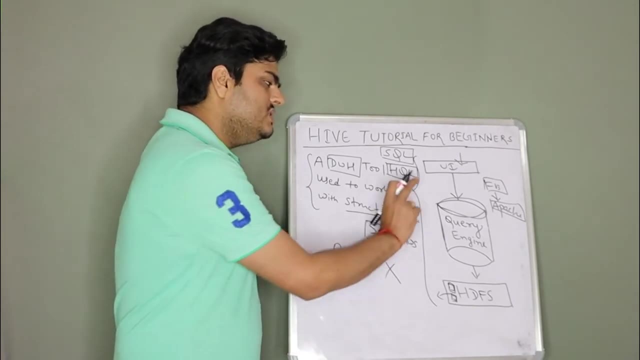 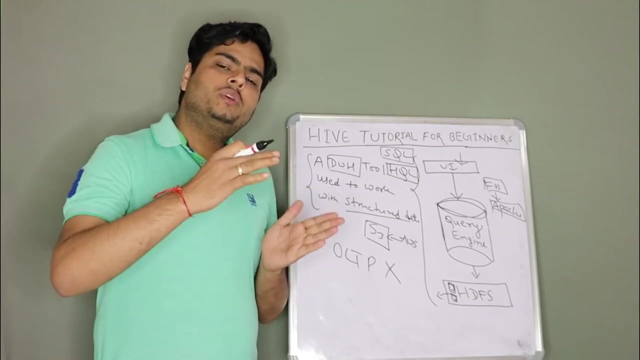 should come from the database immediately. That is, online transaction processing. Hive and normally big data platforms are not supported for that. Okay, What is it supported for? It is supported for batch processing. The meaning of that: in the same superstore, one month of transaction is done, All the one month of transaction you want to push to. 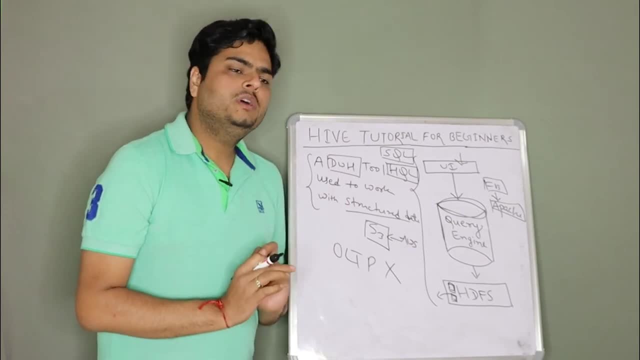 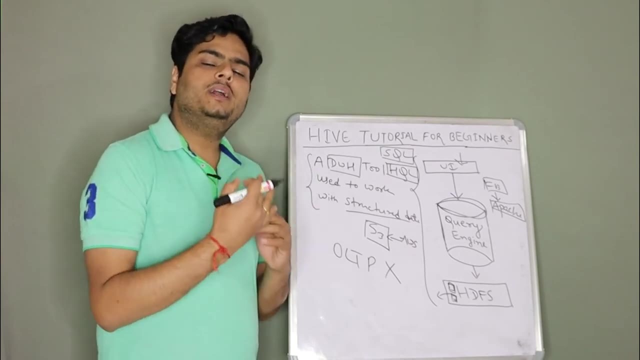 your data warehouse. You want to push to your Hadoop system. That is where Hive is useful. Okay, It will store everything, all the historical data, and it will help you in viewing that, analyzing that, all these things. So Hive is not an OLTP system, Hive is not a real-time. Hive is a